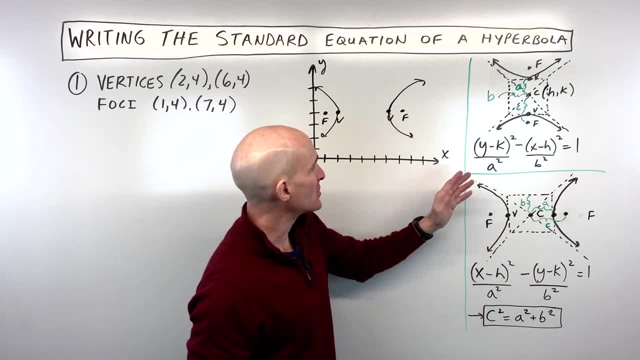 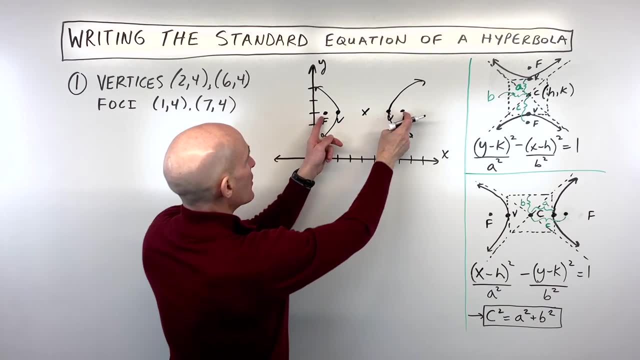 then the y squared term would be written first. And what we can do now is we can find the center point right here, which is halfway between the vertices. it's also halfway between the foci. You could use your midpoint formula or, if you have a good graph, you can just you know count. but let's 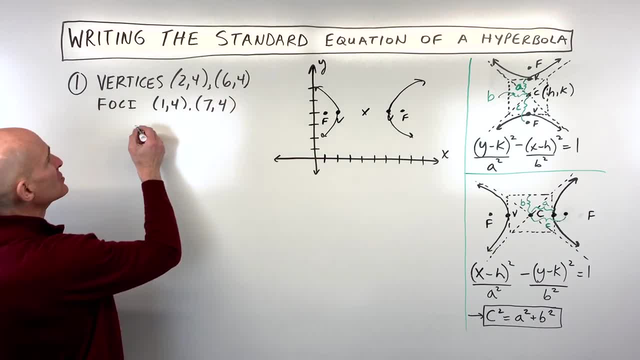 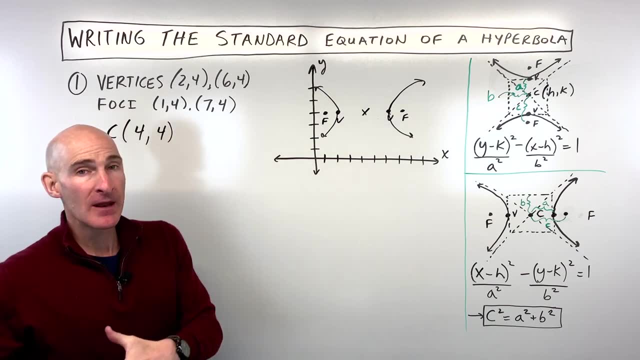 just do the midpoint. So two plus six is eight, divided by two is four, and four plus four is eight, divided by two is four. So that means that our center is at four four. Now when I like to write these equations, I kind of like to piece it together as I go. What I mean by that is: I know. 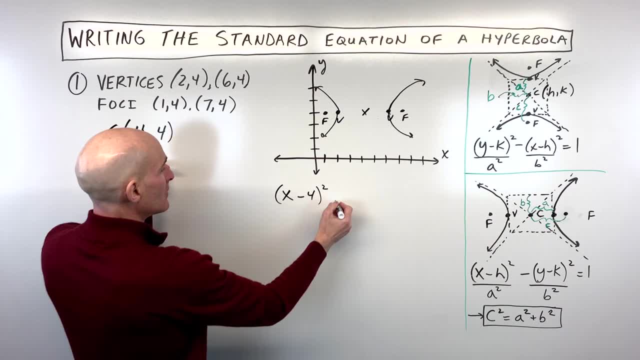 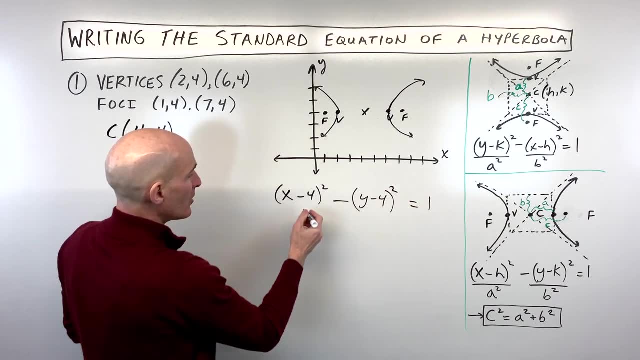 this is going to be x minus the x squared into the center, sorry, and minus the x squared into the, minus y minus our y coordinate of the center. okay, squared, it always equals one for hyperbolas and ellipses, right. but what we have to figure out now are the a squared and the B squared. now what does? 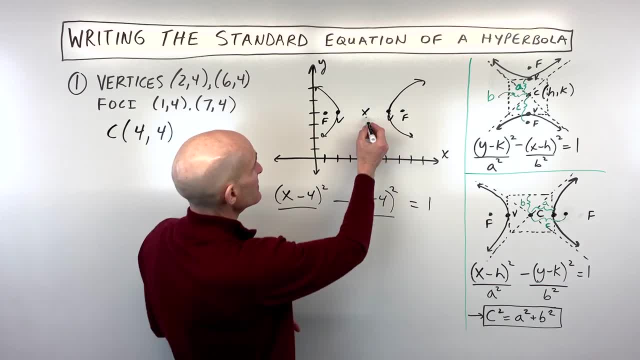 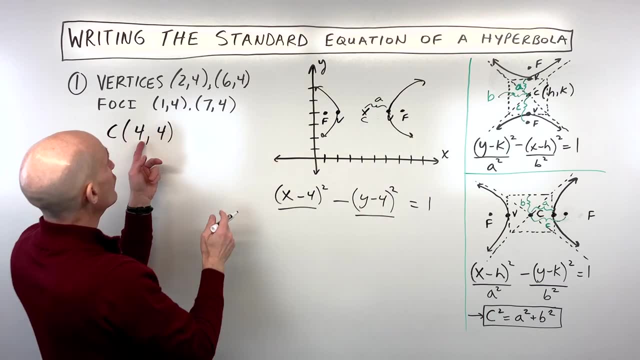 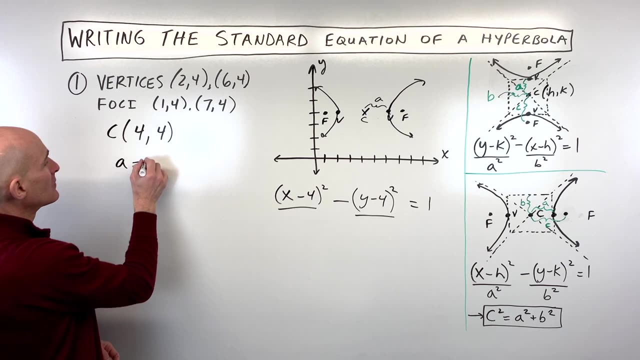 the a squared represent. well, the a is the distance from the center to the vertex. so this is your a, and in this case you can see that's from four. four to six, four. so you can see we're going two units, so our a value is equal to two. let's write that down now. the distance from the center to the foci. 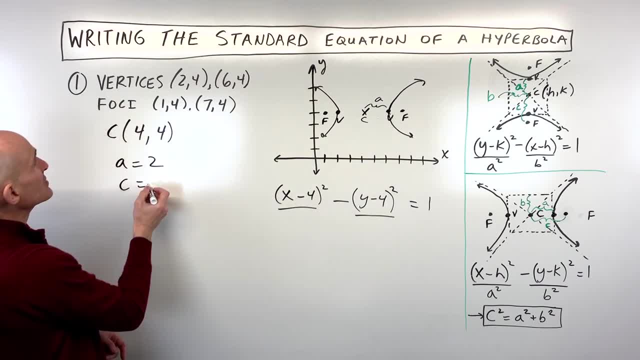 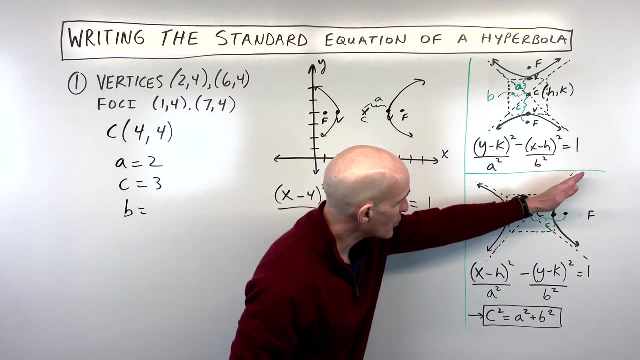 that distance is c, so c is going to be from four. four to seven, four, so that's a distance of three and b is this distance here? okay, when we draw that rectangle, we use the corners of the rectangle to draw our asymptotes. that distance there is b, but there's a formula you want to memorize. 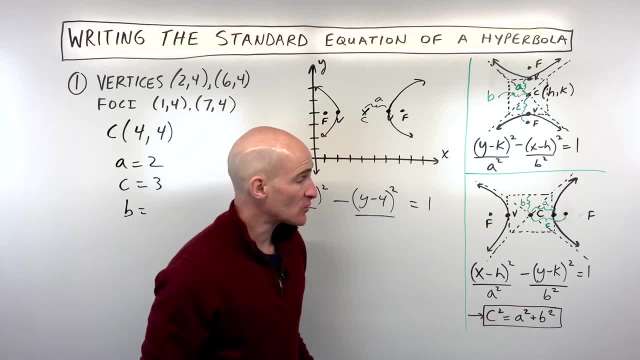 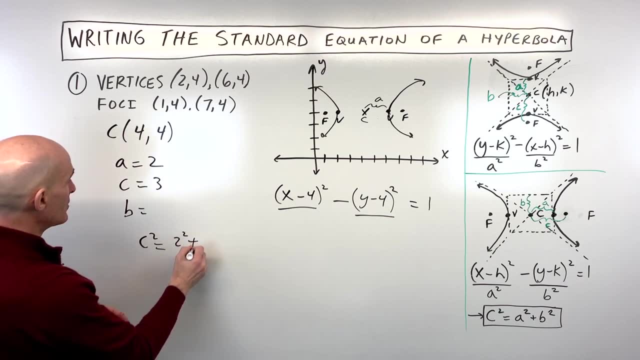 for our asymptotes. so we're going to use the corners of the rectangle to draw our asymptotes for hyperbolas. and that c squared equals a squared plus b squared. so in this case to solve for b, we have: c squared is equal to a squared, which is two squared plus b squared is equal to. 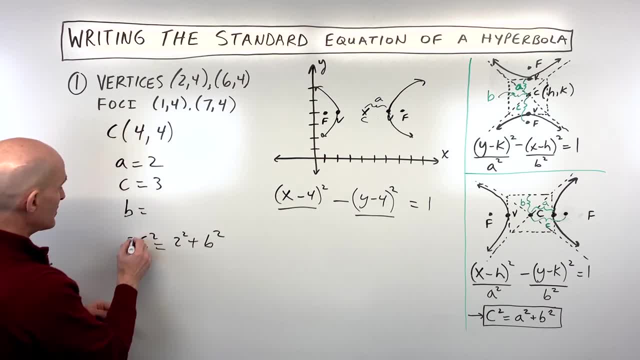 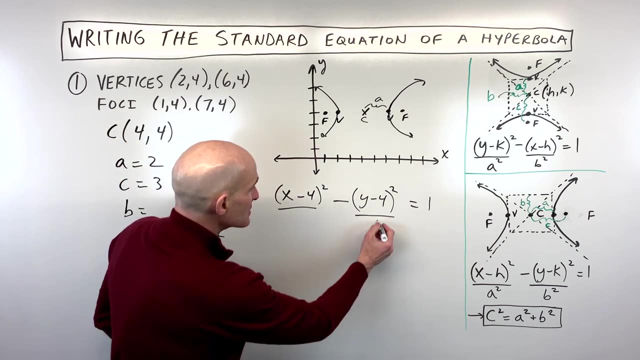 c squared, and c squared, we know, is three. so let's change this to three squared, so that comes out to nine, equals four plus b squared. subtract four from both sides and you can see that b squared is equal to five. so we can see in our equation here: b squared is 5, a squared is 2 squared, which is 4, and you've got 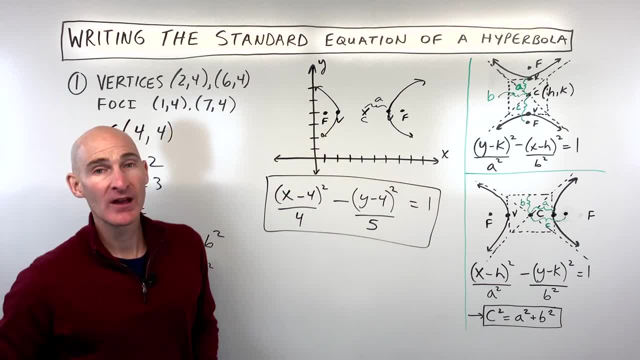 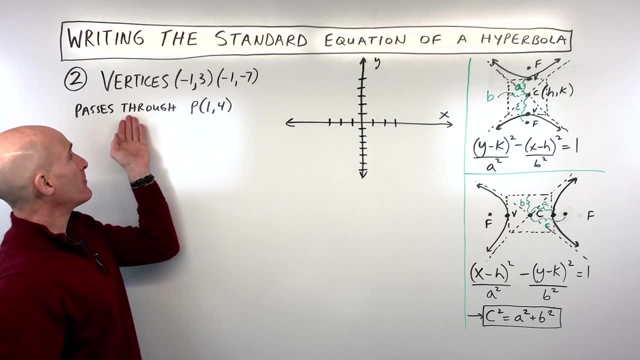 the equation of your hyperbola in standard form. Let's take a look at another example. Okay, example number two is a little bit different in the sense that they're giving us the vertices and a point that the hyperbola passes through. So how do we get the standard form of the equation of this? 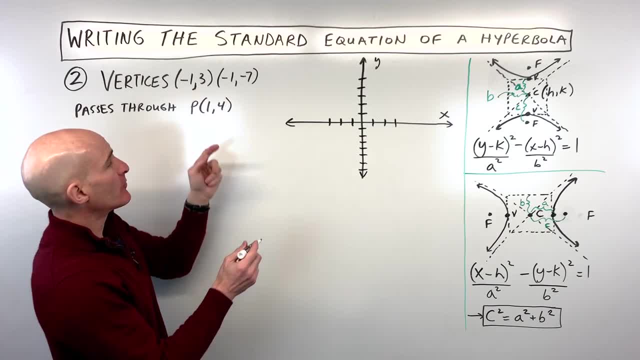 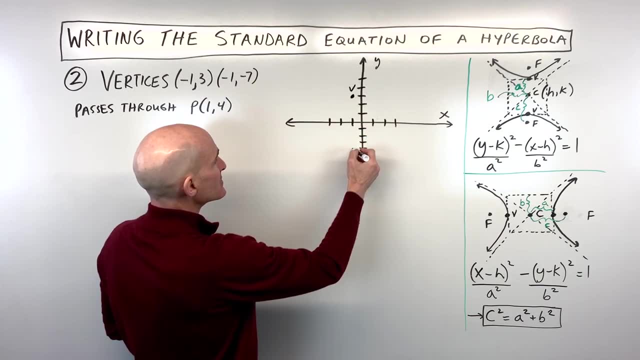 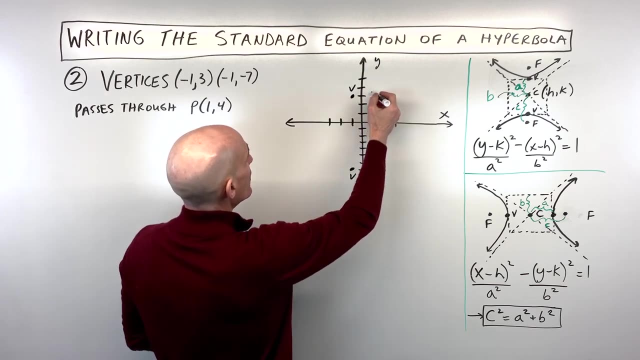 hyperbola. Again, I would recommend drawing a sketch. We've got the point negative 1, 3, which is going to be one of our vertices, and the other one is at negative 1, negative 7, which is right about here, And you can see that the point that it's going through is 1, 4, right about here. So 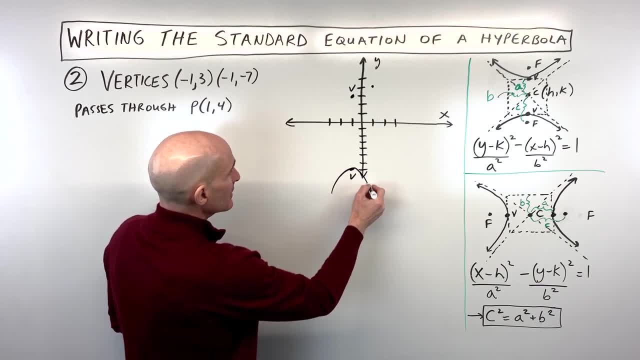 what this tells us is that the graph is going to be opening in the what I like to call the y direction, basically up and down. okay, in this vertical direction, which means it's going to be opening in the y direction. So we're going to be opening in the y direction, basically up. 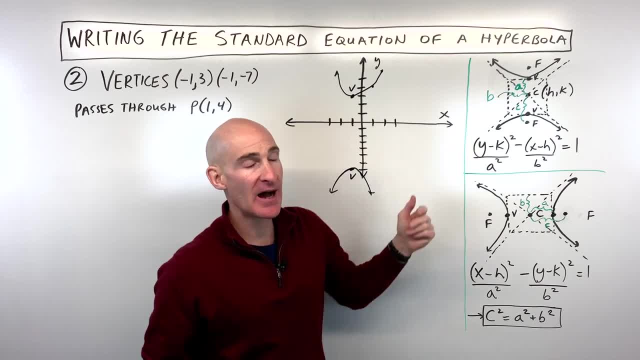 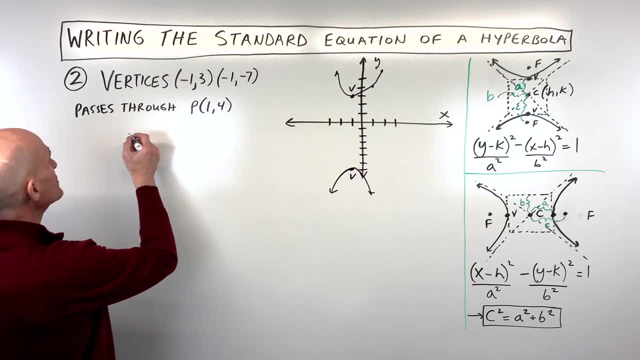 and down. So we're going to be opening in this form right here. where the y squared term comes first, It's the positive term. So the next thing I'd like to do is maybe find the center point, and the center is halfway between the vertices, So you can use the midpoint formula or you can. 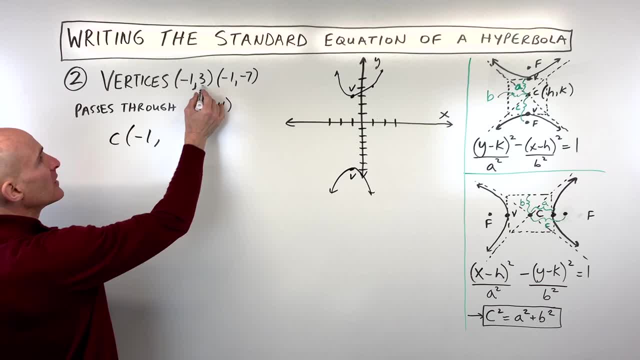 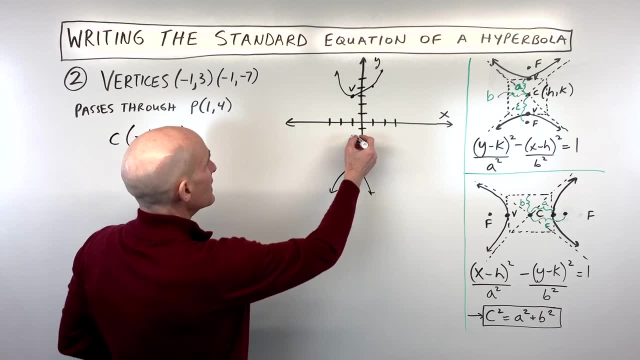 just count on your graph. So it looks like this is going to be at negative 1, negative 4 divided by 2 would be negative 2.. So basically, just add the x's and divide by 2, add the y's and divide. 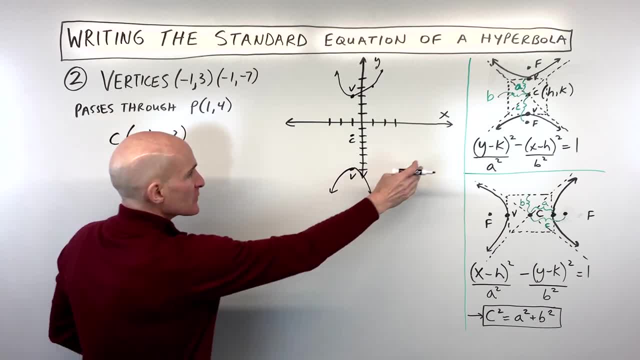 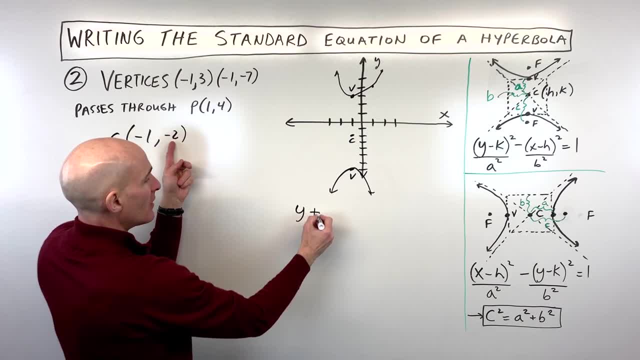 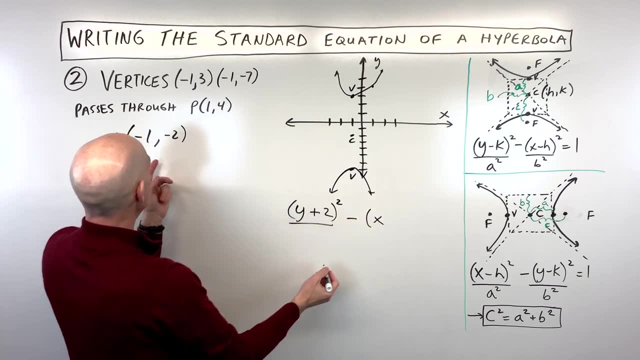 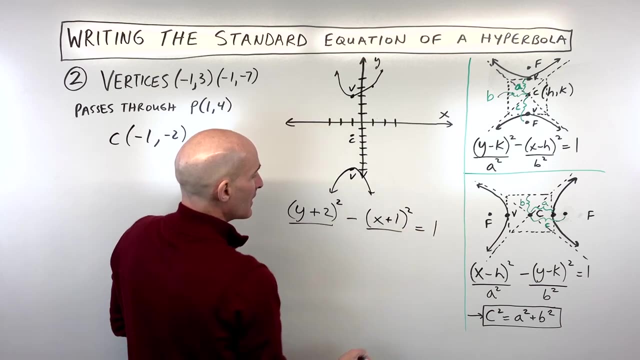 y minus the y coordinate of the center, So that's going to be y minus negative 2. or y plus 2 squared minus x minus the x coordinate of the center, So that's going to be x minus a negative 1, which is x plus 1 squared, and hyperbolas always equal 1.. Remember the distance from the center to 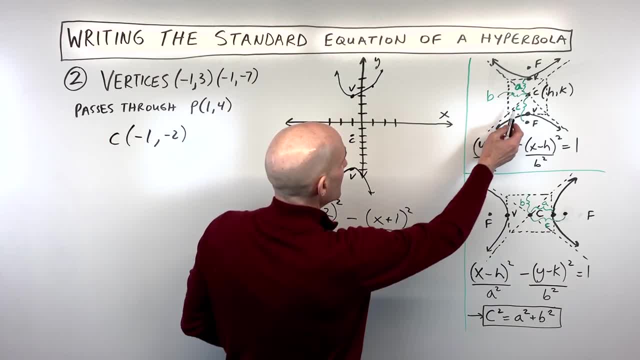 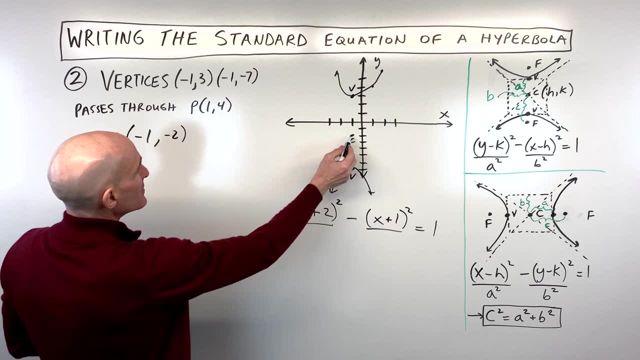 the vertex. that distance we call a okay distance from the center to the vertex, and so that is going to be a squared as our denominator. So here, a is the distance from- let's see, negative 2. okay, to negative 7, that's a distance of 5.. So our 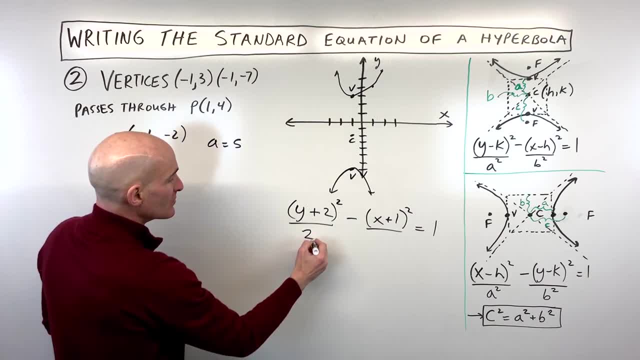 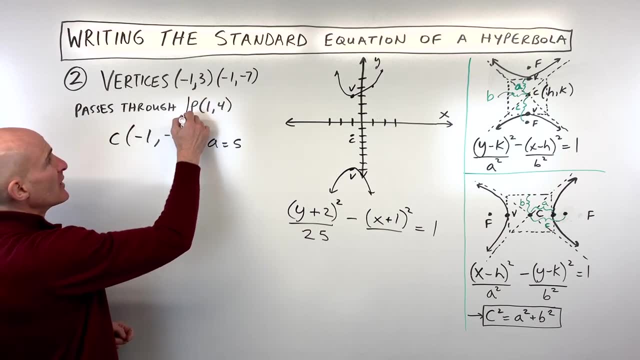 a value is equal to 5.. So 5 squared is going to be 25.. All we have to do now is solve for our b squared, and that's where this point comes into play. So we know it goes through the point 1, 4.. 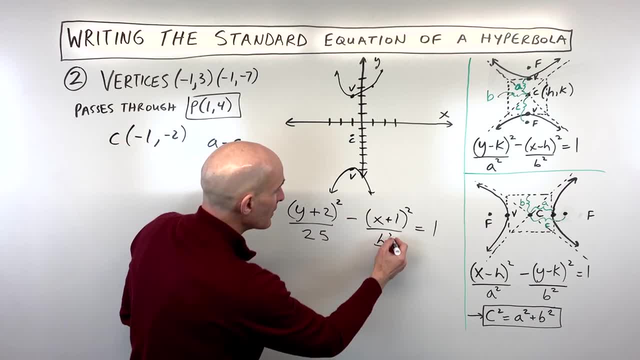 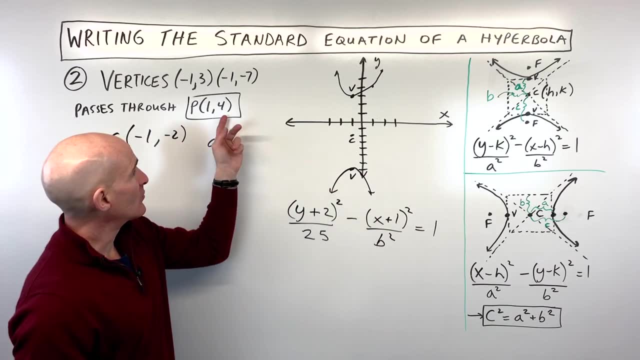 If 1,- 4 is a point on our equation, here on our graph, then it's going to make this equation true, right? So what we're going to do is we're going to replace 1 for x and we're going to put 4 in for y and we're going to solve for our b squared. So let's go. 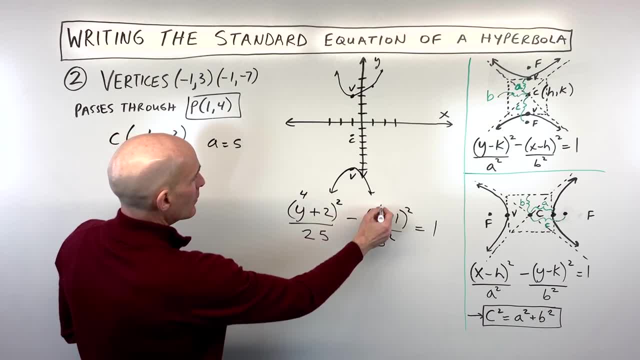 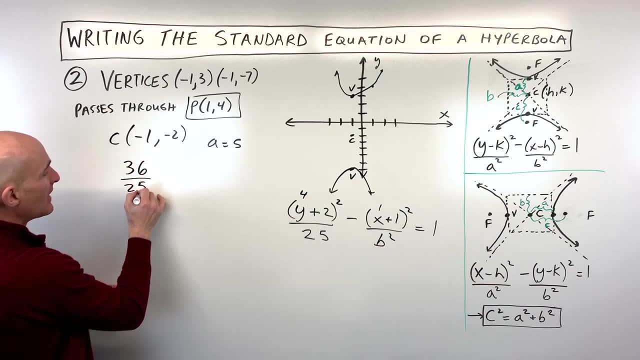 ahead and do that. So if I put 4 here and 1 here, what do we get? We get: 4 plus 2 is 6.. 6 squared is 36 over 25 minus 1 plus 1 is 2.. 2 squared is 4.. So that's 4 over b squared is equal to 1.. Now 1. 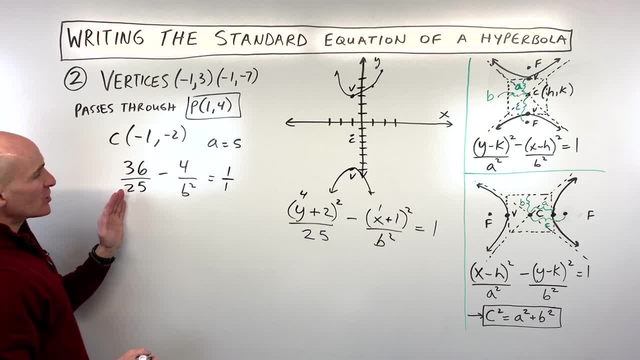 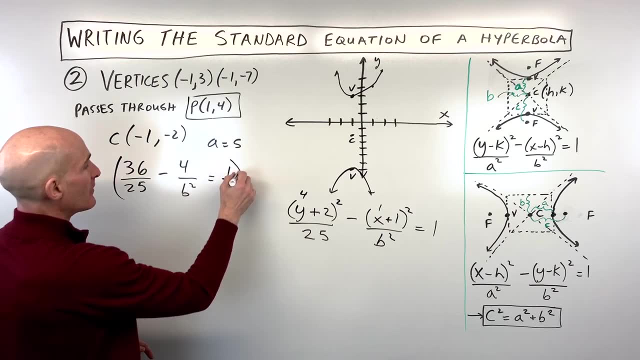 is like 1 over 1, right? So what we could do here is we could actually clear the denominator by multiplying through by the common denominator, which is 25 b squared. So let's go ahead and do that: Multiply our whole equation by 25 b squared. If we do that here, this is going to. 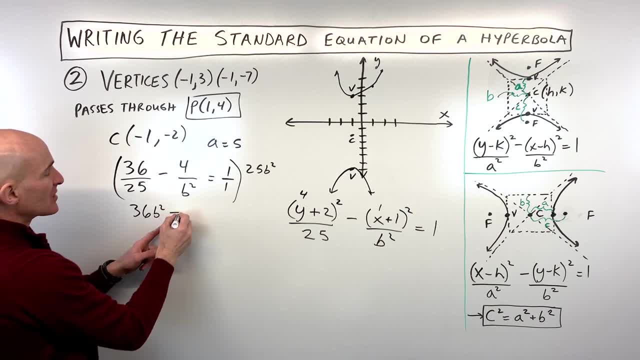 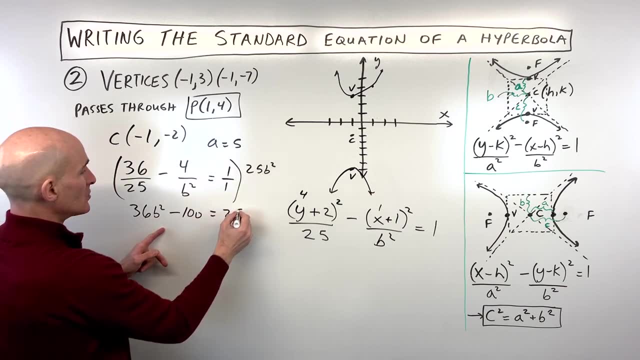 come out to 36 b squared, This is going to come out to minus 100, because you can see the b squareds cancel 25 times 4 and this is going to come out to 25 b squared. So if I subtract 36 b squared, 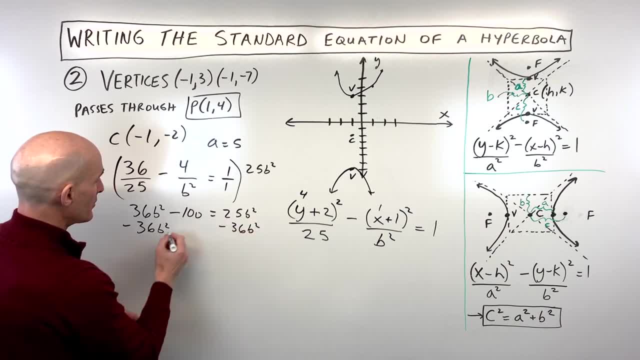 from both sides to get the variables on one side, numbers on the other. That's going to come out to negative. 100 is equal to negative 11, b squared. Divide both sides by negative 11.. So you can see that b squared is coming out to 100 elevenths. So we can replace: 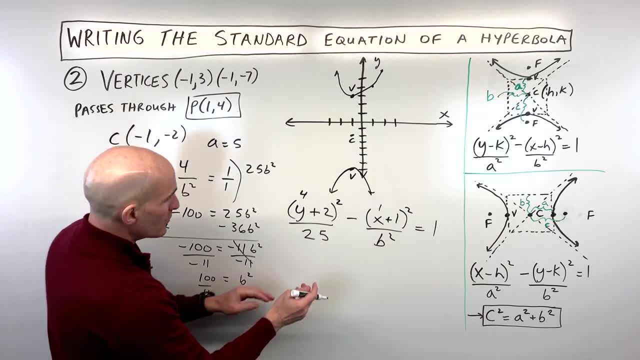 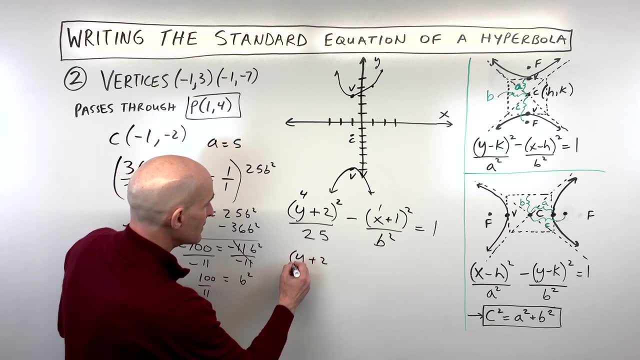 b squared with 111ths, or when you put 111ths in here, when you divide by a fraction, it's like multiplying by the reciprocal. So if you want to write this kind of as a neat form of the standard form of the equation of our hyperbola, 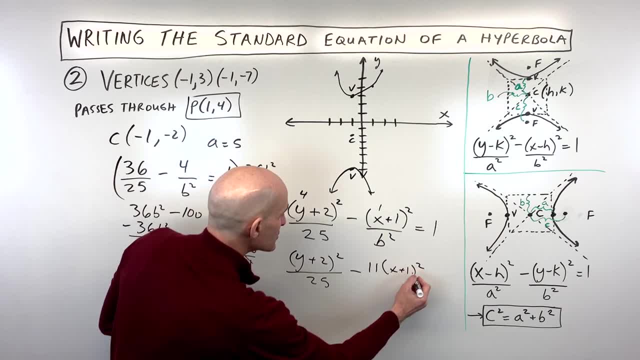 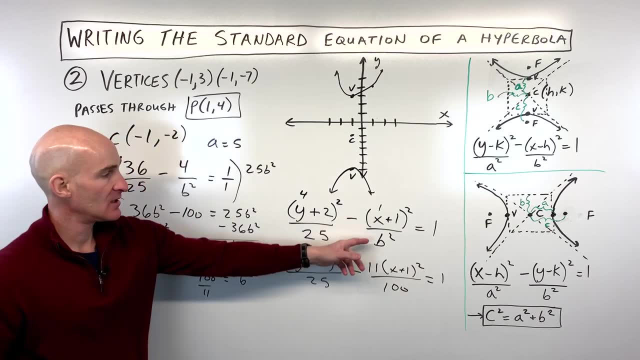 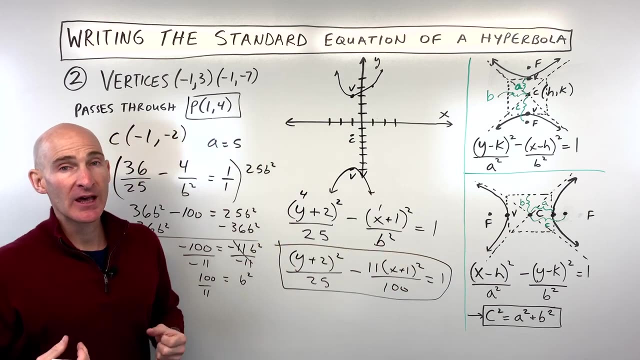 Really look like 11 x plus 1 squared over 100 equals 1.. Or if you don't like that, you can just write the 111ths in the denominator and it's okay to have that fraction there. But this is just a little bit kind of rewritten a little bit neater. So let's take another look at a different example. 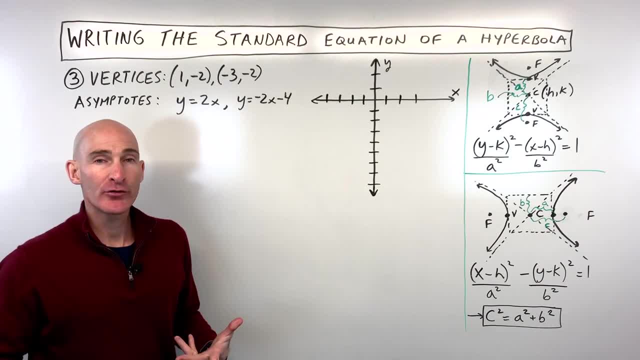 in number three Before we dive into example number three. if you're enjoying my channel and you come back to see my videos now and again, consider supporting the channel. by joining as a channel member, You can help support the content that I'm putting up here and I really appreciate it. 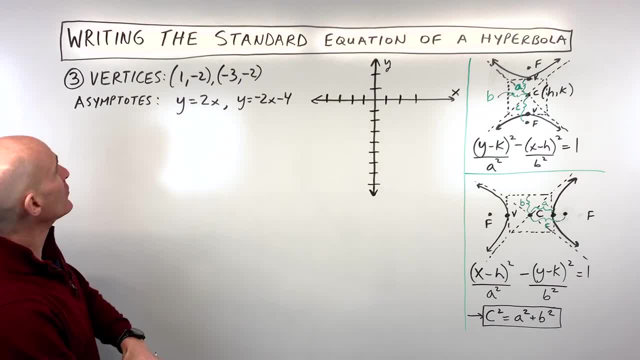 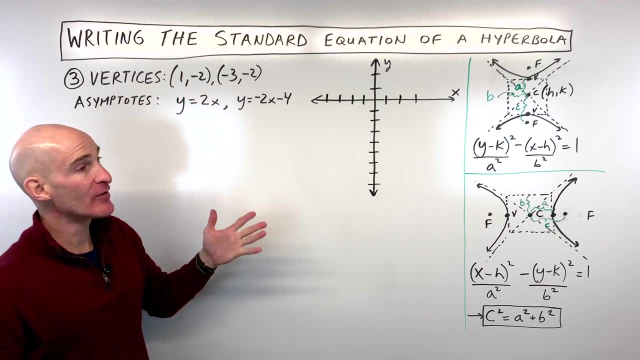 Let's take a look at this last example, though. See if you can do this one on your own. This one's a little bit different than the first two, in the sense that they're giving us the asymptotes and the vertices. So how do we find the standard form of the equation of this hyperbola? 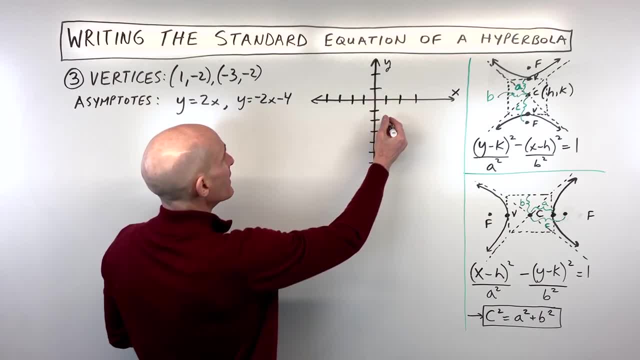 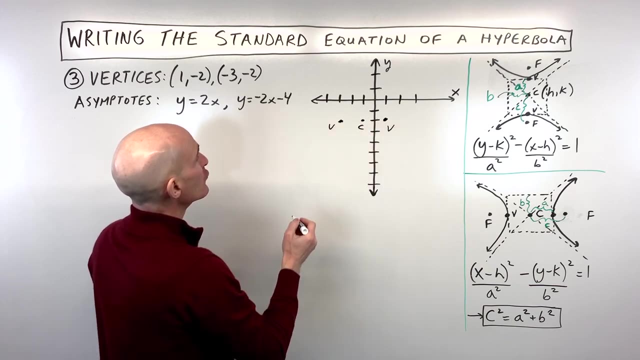 Again, I would start by drawing up a little sketch so we can see one negative two is right here and negative three negative two is right here. So those are our vertices And we know that the center is halfway between the two vertices, So you can do your midpoint formula. 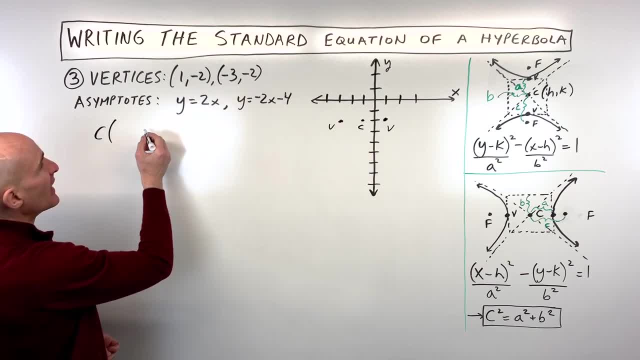 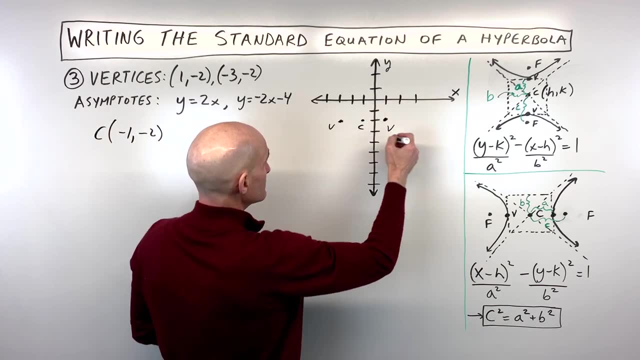 or you can just count. So in this case it looks like it's going to be at negative one, negative two, So it's just halfway between, and we know that this hyperbola is going to be opening in the horizontal direction, or what I like to call the x-direction. 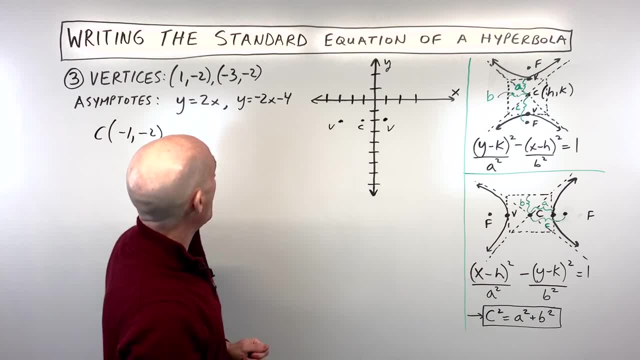 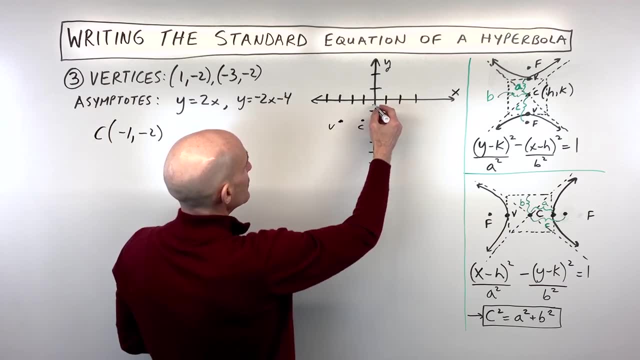 So it's going to be in this form right here. So now what we're going to do is: let's go ahead and graph the asymptotes. graph the asymptotes, So y equals 2x is going to be going through the origin and has a slope of 2.. 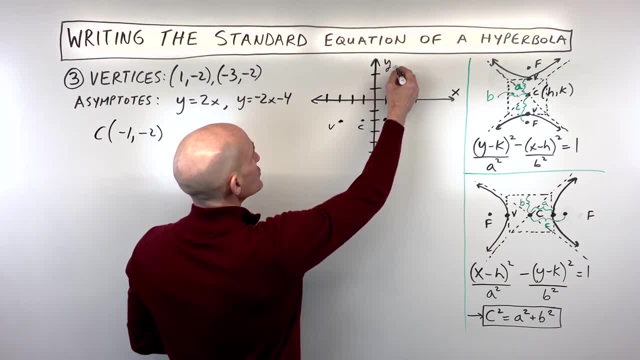 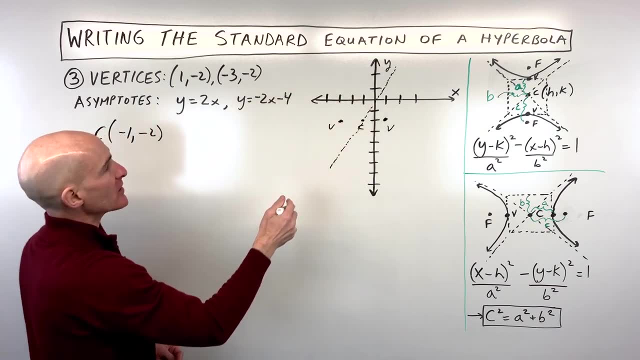 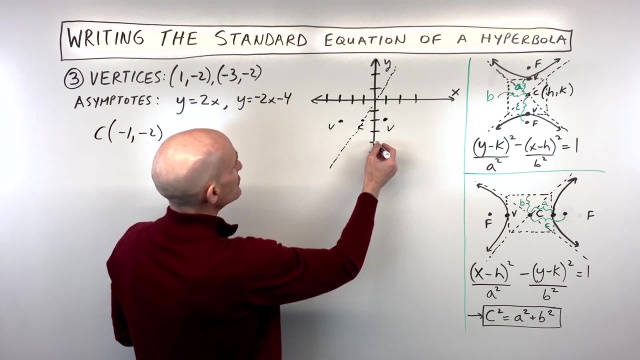 So rise 2, run 1. And the asymptotes will also pass through the center point of the- you know hyperbola. So that's important. And then over here the y-intercept is negative 4.. Let's see 1,, 2,, 3, 4 and has a slope of negative 2. So that's going to be going something like: 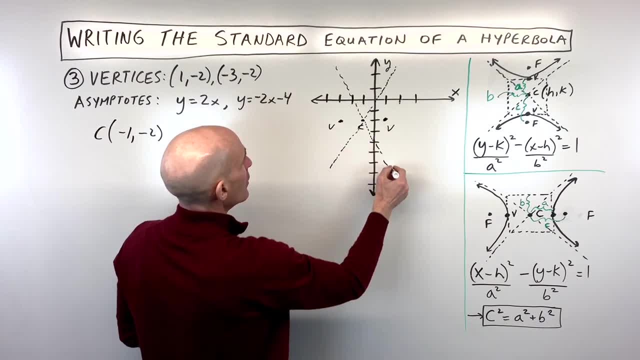 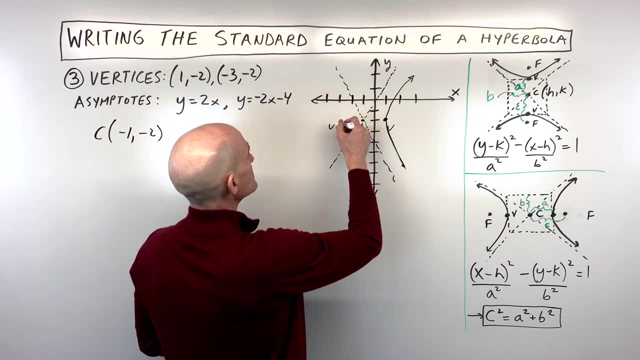 this. Okay. so now we have a rough sketch here and you can see that the hyperbola is going to look something like this where it approaches those asymptotes. Okay, roughly like that. So let's go ahead and piece together what we have so far. So we know. 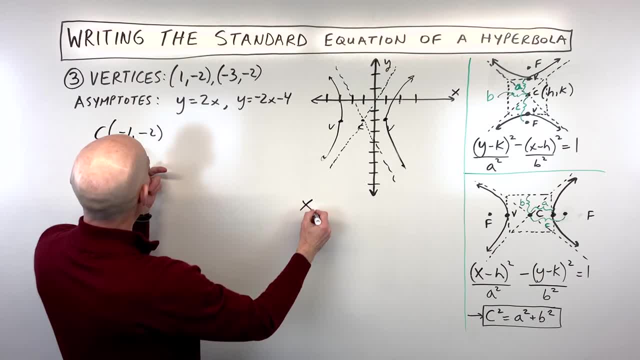 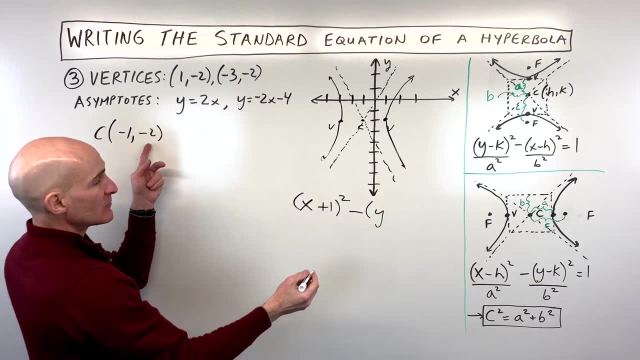 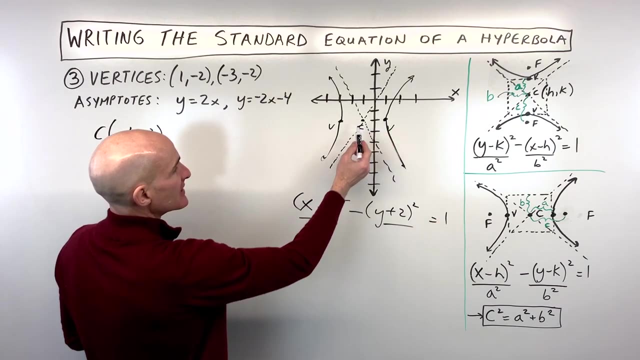 it's in this form. We know the center, So this is going to be x minus negative 1, or you could say x plus 1 squared minus y minus negative 2, or you could say y plus 2 squared Equals 1.. And remember the distance from the center to the vertex. that distance is a.